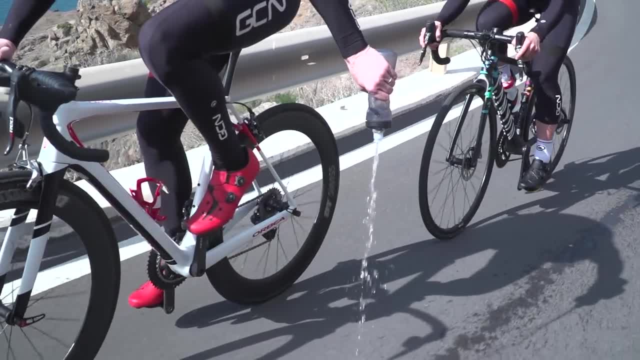 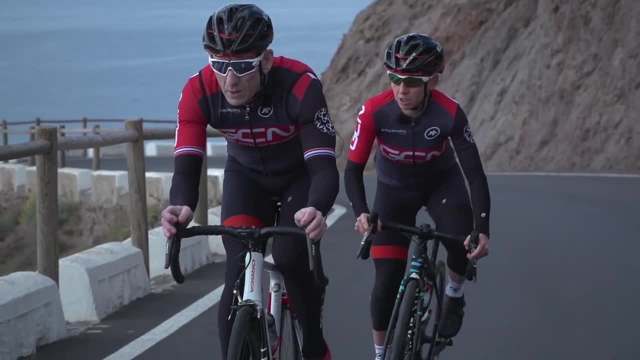 I should say: only do that if it's definitely spare, because running out of water on a long climb will not make you faster. Also, tuck in out of the wind. It doesn't make such a difference on a climb when you're going slower, but it still helps. Also, make sure you look. 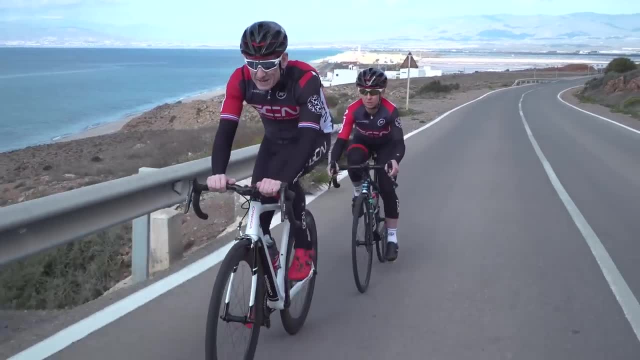 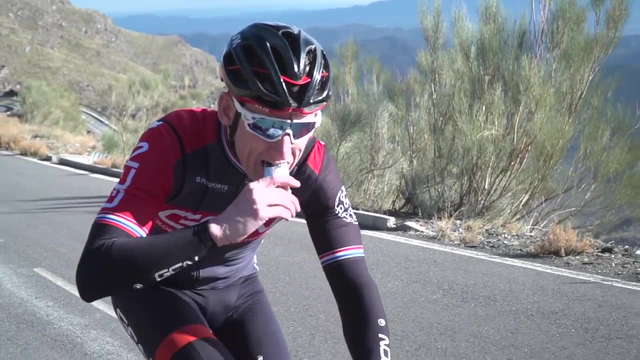 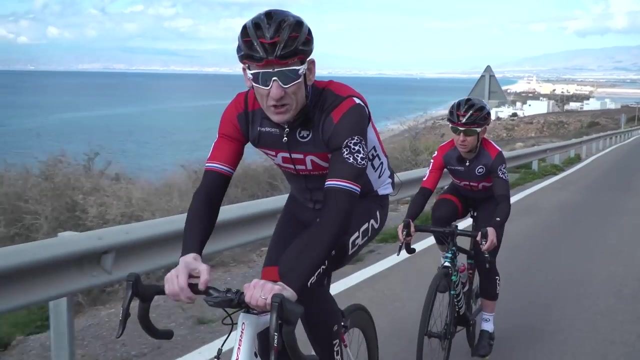 after your body. So look at your fueling strategy. Make sure you're eating enough Plenty of carbohydrate, little and often, So don't stuff your face, Otherwise you simply won't be able to breathe properly on the climb. And the same can be said for hydration as well. Make sure you're drinking little. 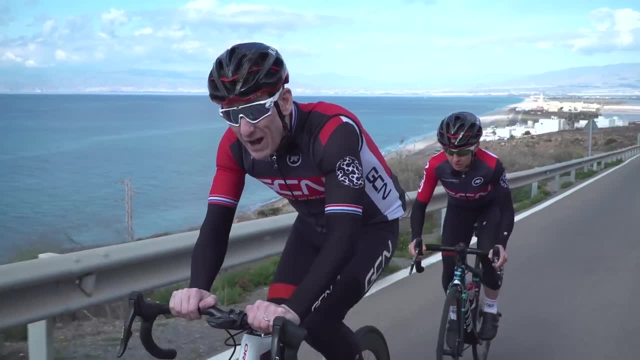 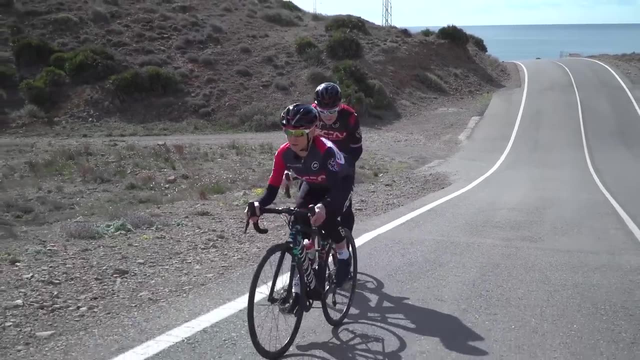 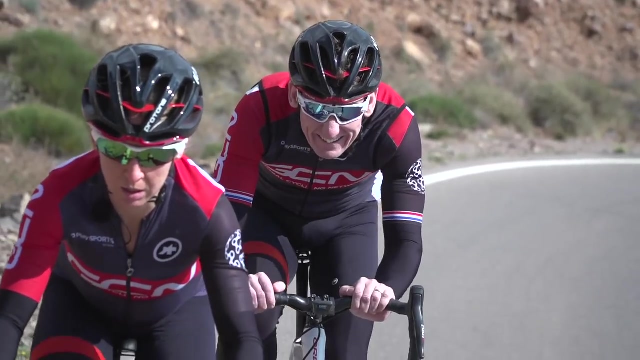 and often, and making sure you don't overheat, Because if you overheat, that will rob you of really valuable energy. Now to what I think truly makes a tough rider someone who can push themselves to hang on on a climb. First and foremost, embrace the challenge. 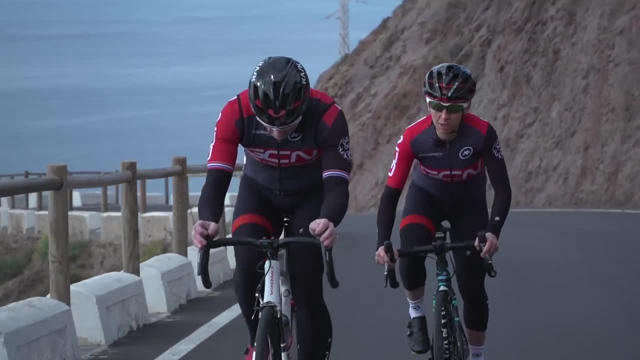 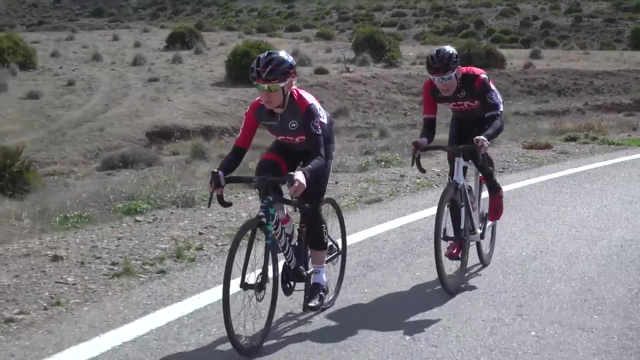 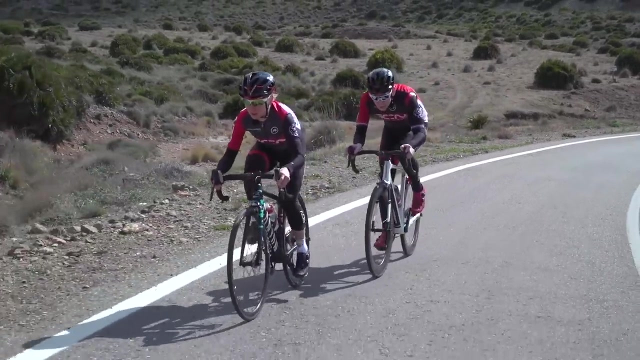 Now it's going to be really hard and super tough to try and hang on to the wheel of a rider that's stronger than you on a climb, but just accept it and suffer. In fact, riding like this and holding on to stronger riders on climbs will make you a stronger rider as. 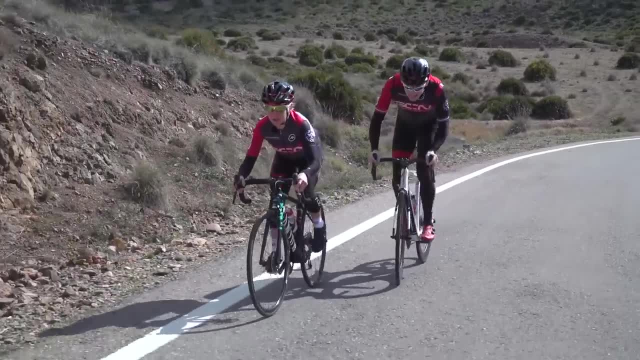 well. So simply embrace it, Try to make the pain your choice and be happy about it because, let's face it, cycling is a sport where you'll have to suffer a bit if you want to improve your fitness, So you'll. have to make the pain your choice and be happy about it because, let's face it, cycling is a sport where you'll have to suffer a bit if you want to improve your fitness. So embrace it. Try to make the pain your choice and be happy about it because, let's face it, cycling is 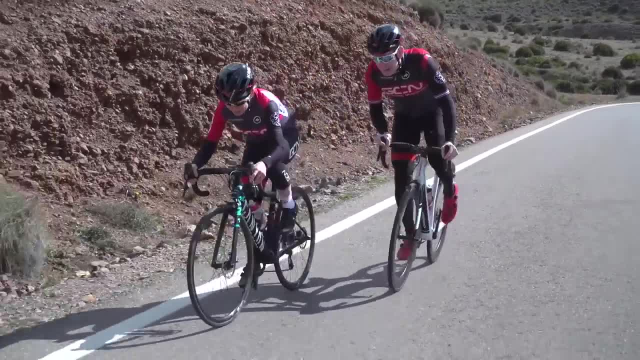 a sport where you'll have to suffer a bit if you want to improve your fitness. Emma, you like making me suffer, don't you? Oh, I'm suffering too. When are we allowed to slow down? Oh, I'm suffering too. When are we allowed to slow down? 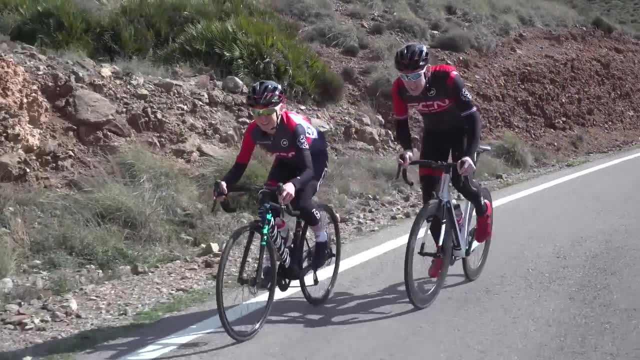 Now No excuses. If you start giving yourself a get-out clause, the chances are you'll use it. And I'm not saying that it's not okay to get dropped, but you know, if you're tired or overtrained or it's not the riding you were supposed to be doing that day, but just 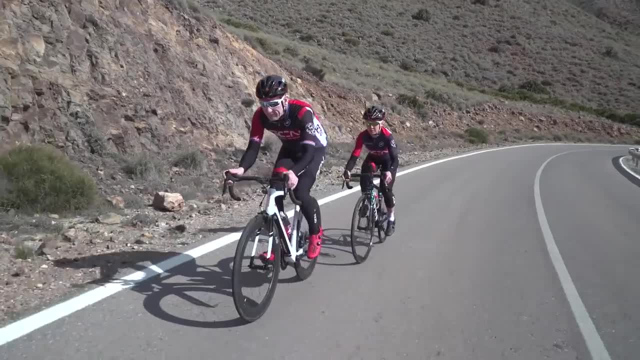 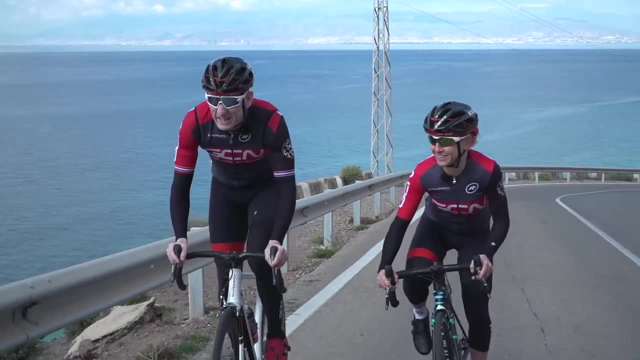 be sure that it's a real reason and not an excuse. No excuses. If you start giving yourself a get-out clause, the chances are you'll use it, And I'm not saying that it's not okay to get dropped, but you know, if you're tired. 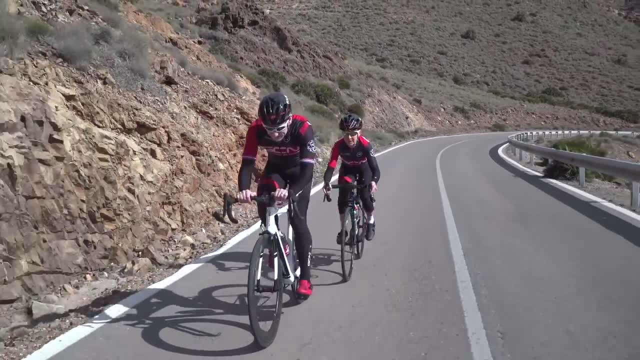 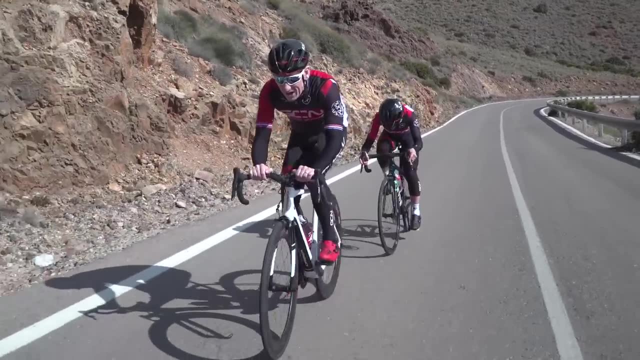 or overtrained or it's not the riding you were supposed to be doing that day. but just be sure that it's a real reason and not an excuse. Yeah, because once you're dropped from the group it's going to be a lot harder to get. 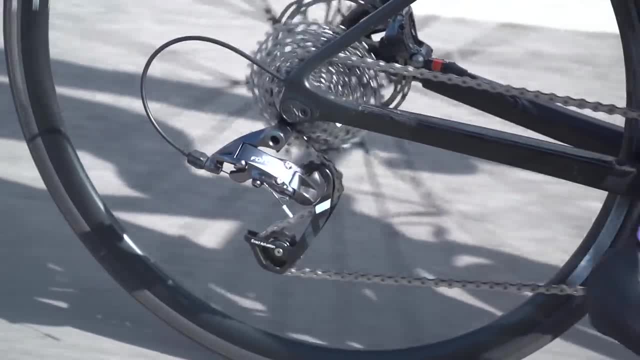 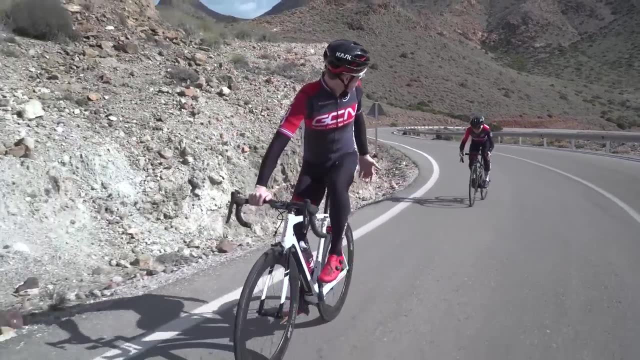 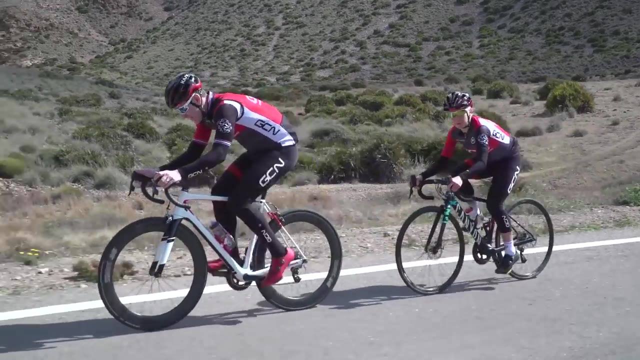 back on again. So a heavy bike or a rubbing brake, well, that's no excuse to lose that wheelie of you. Come on, Come on. blimey Motivation, How bad do you want it? Why Note that the level of your motivation does not? 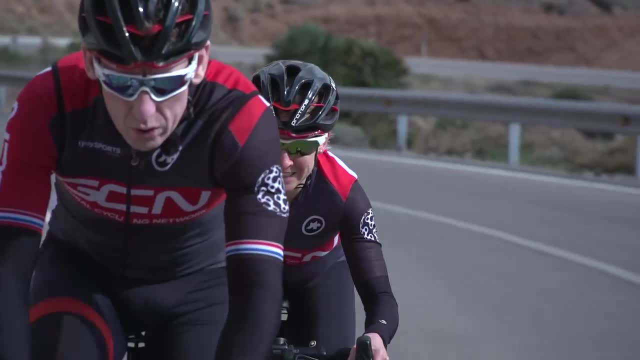 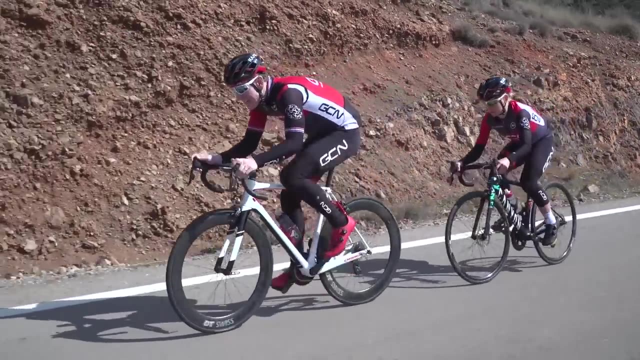 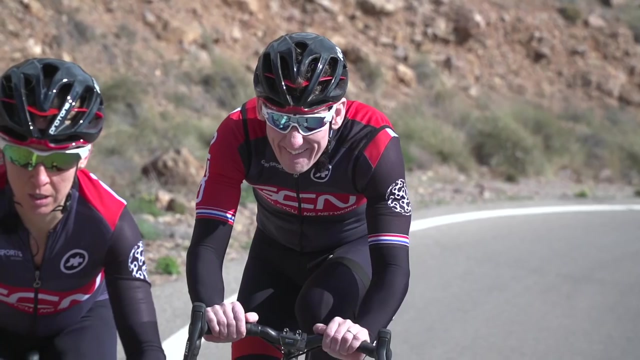 necessarily have to be proportional to the significance of the actual situation. Now I've seen riders turn themselves inside out on a pointless training ride. Now, that is a skill and it can be learnt. Practice to ride like you care. Don't focus on the pain. This actually makes it harder to bear To distance yourself from. 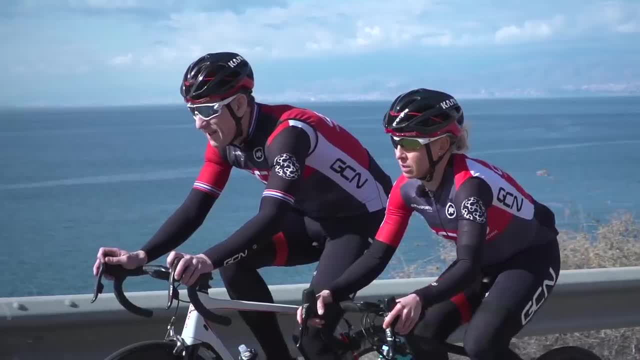 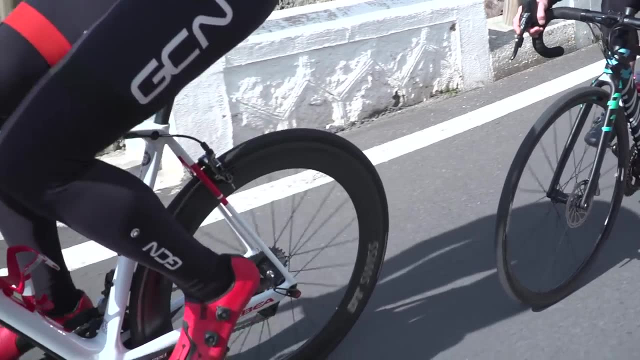 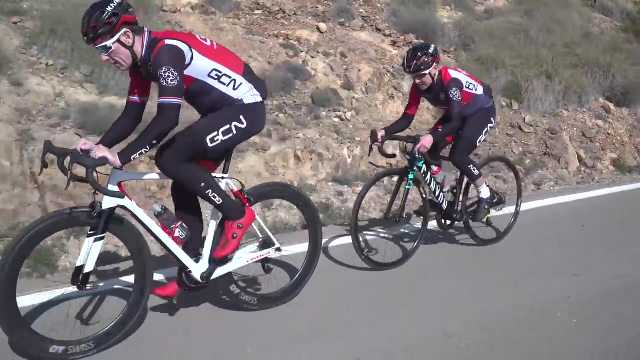 discomfort, distraction can work for some. Soak in the view of the beautiful mountains, or focus very hard on the rider's back wheel in front of you, Or think about cake. Watch the wheel in front and really focus on not letting go. It's surprisingly effective. Of course, don't just watch the wheel because you don't want. 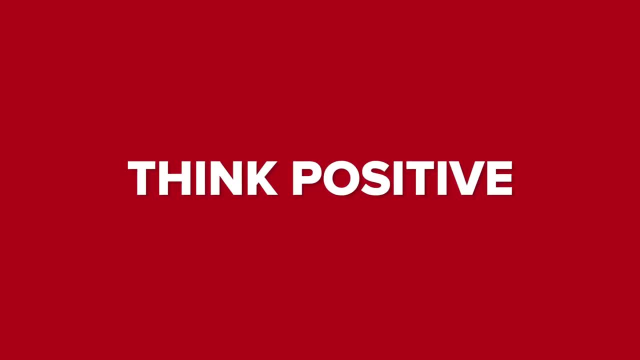 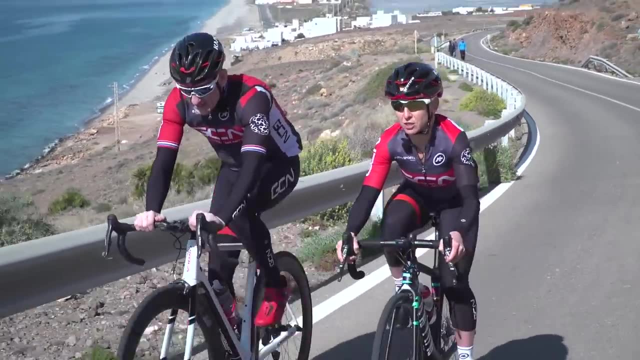 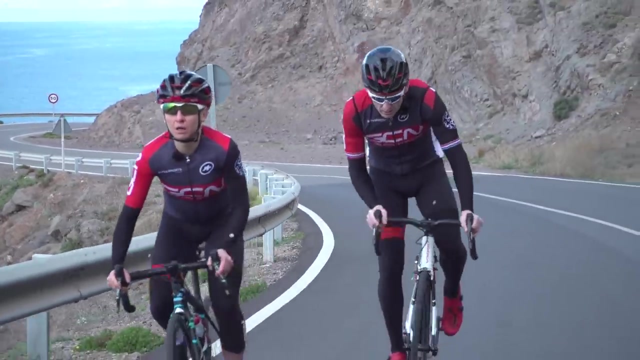 to ride off the road or crash. Think positive. Now this might sound alarmingly new age and hippy, but there is real scientific evidence that shows that being overly self-critical can damage your physical performance. So don't dwell on the fact that maybe your training didn't go very well or everybody else just. 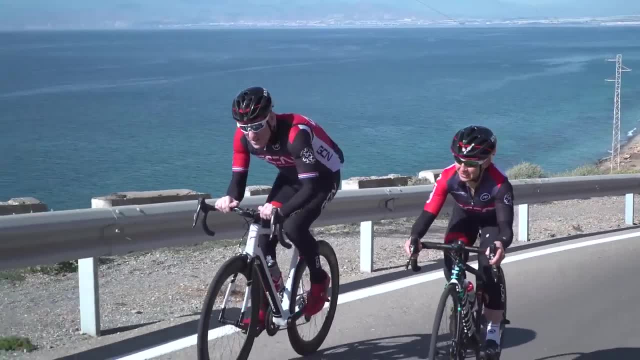 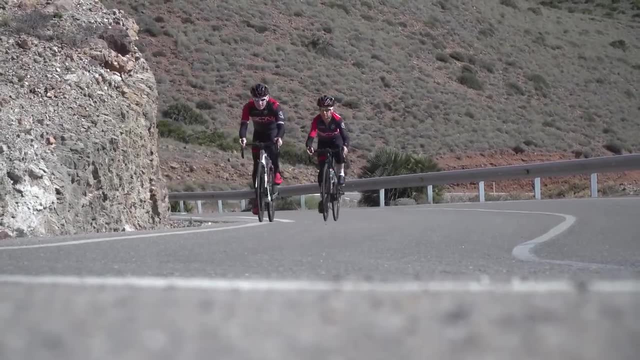 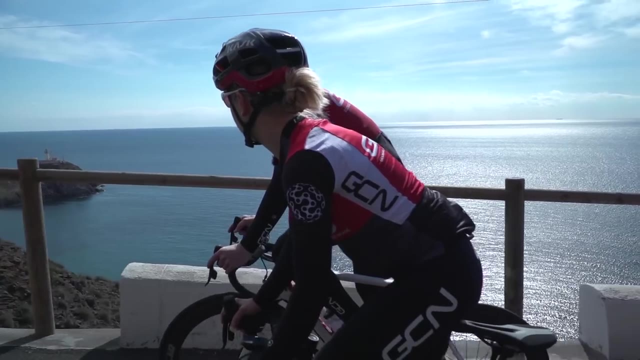 seems so much fitter. Instead, think positive. Think that every moment that you're hanging on to a group of stronger riders that it's actually a real achievement and it's making you fitter and faster. Or if that doesn't work, go back to admiring the view. Or if that doesn't work, go back to thinking about. 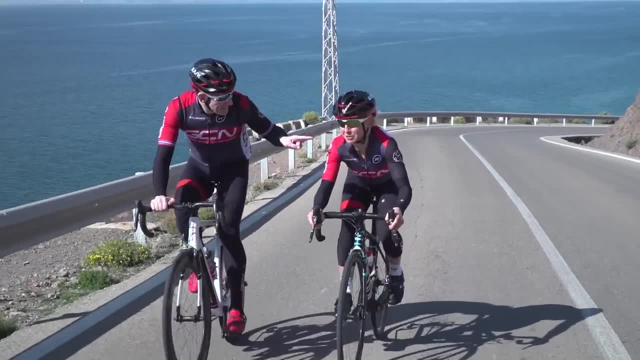 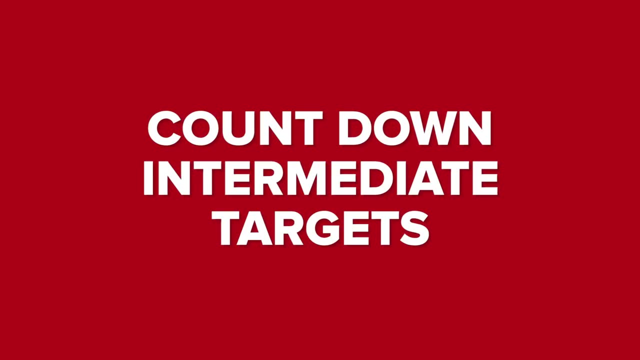 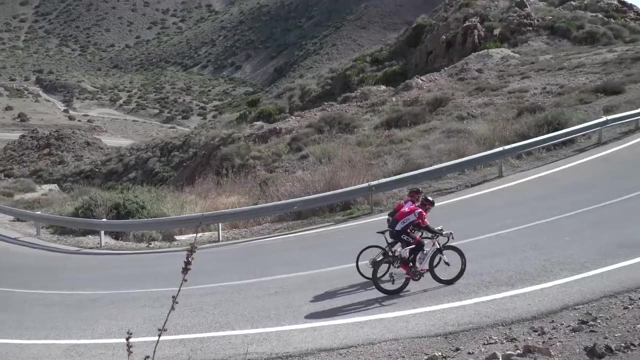 cake. Are you thinking about cake? Possibly, Possibly. That's your cake face, isn't it? Yes, Emma's cake face, Chocolate face too. Hang on for just one more hairpin, Or just one more kilometre, Or just one more minute. 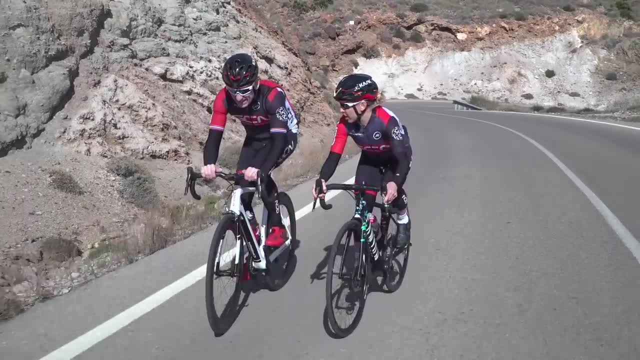 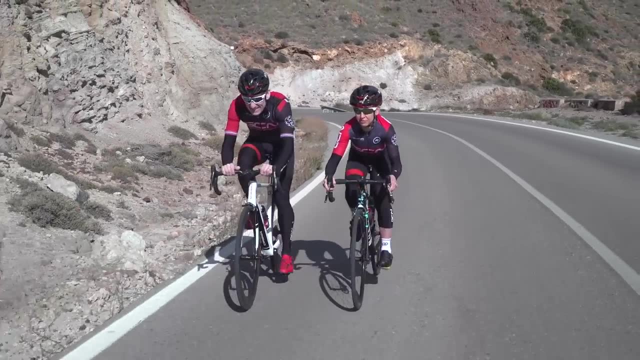 Sometimes the others might have set off too hard and they might ease up or even blow up. I mean, you can't count on it, but it's worth hanging on just in case, because it is so satisfying when it happens. It is, isn't it? 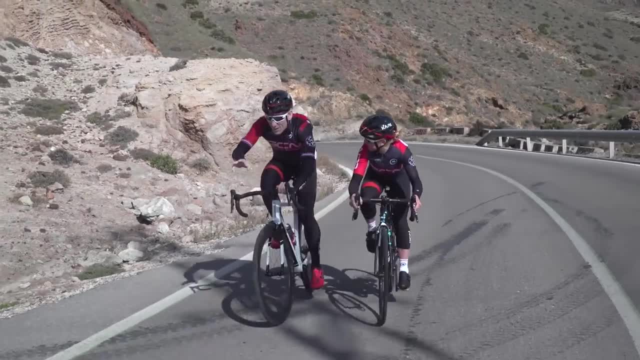 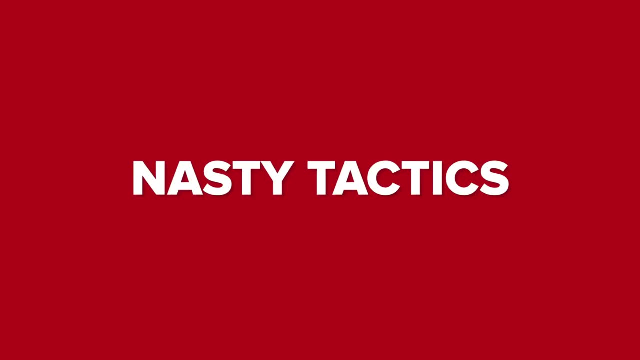 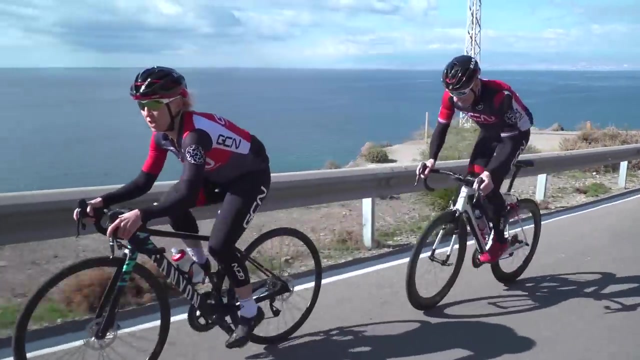 Are you blowing up yet Just one more hairpin? No, I'm just. I'm nearly there. I'm thinking about cake, Oh cake. Be prepared for nasty tactics If the rider in front of you starts putting in surges, or 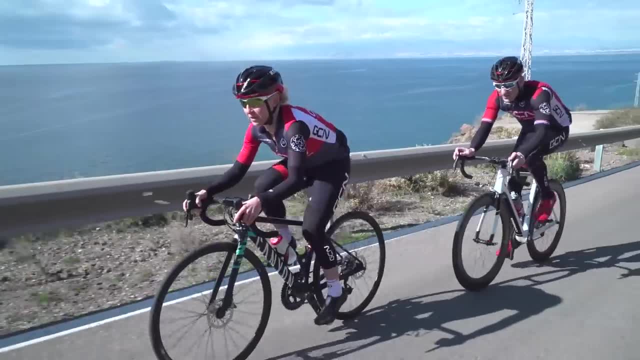 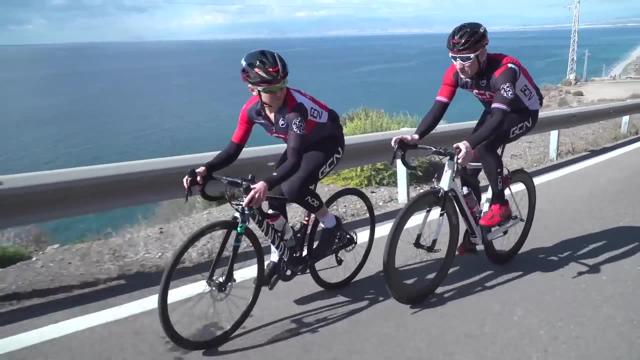 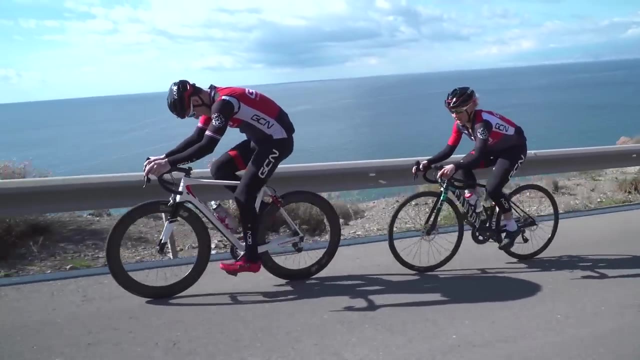 maybe starts chatting cheekily. just hang on. They're testing you, Yeah, because if their tactics don't work on you, it can be very off-putting for them. Sometimes the best form of defence is attack, Or it might just be the racing equivalent. 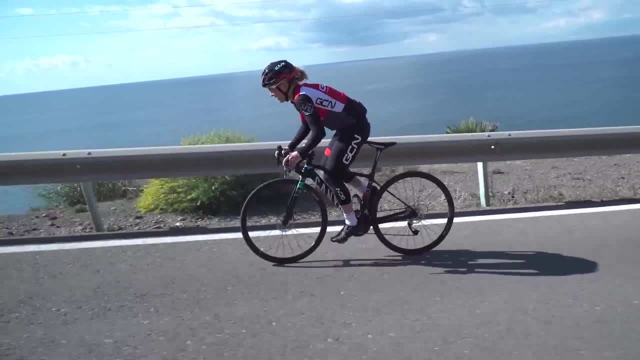 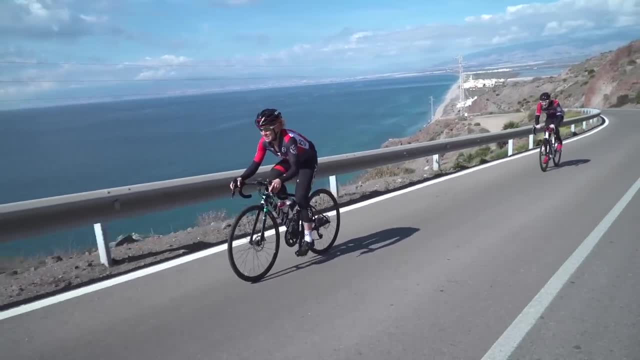 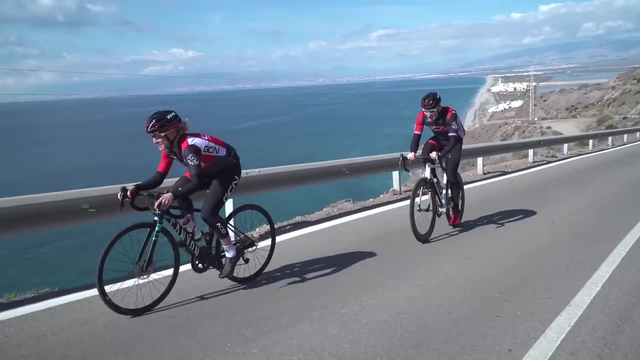 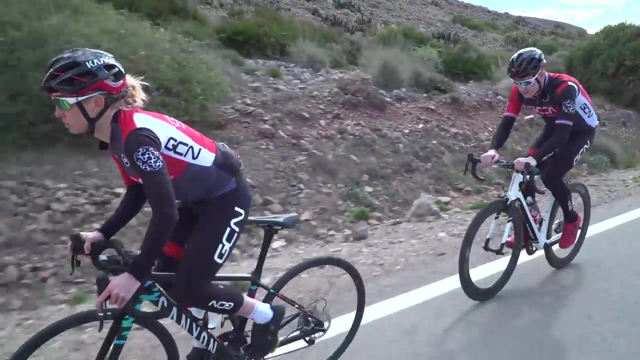 a day. Just don't go down without a fight, or it simply could be that the right buddies you thought was super strong, The bluffing Oh man. Now, obviously you can still use these tactics even if you've done all your training and 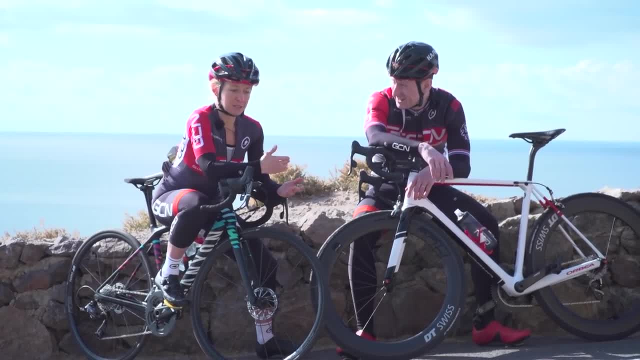 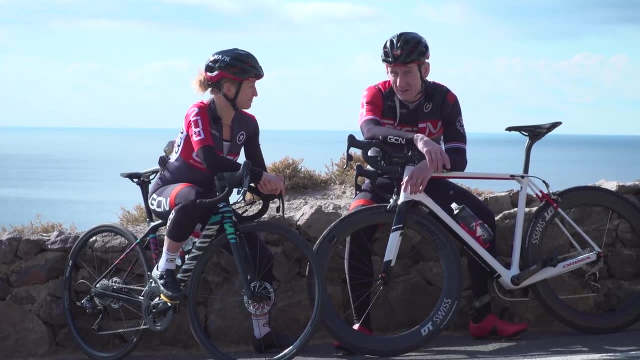 maintained a sensible caloric balance, Like my model athlete, because it'll still help you to hang on to athletes who are stronger than you and ultimately get stronger yourself. Well, that was how to hang tough on a climb: Sticking with climbing. how about clicking just down here for six? 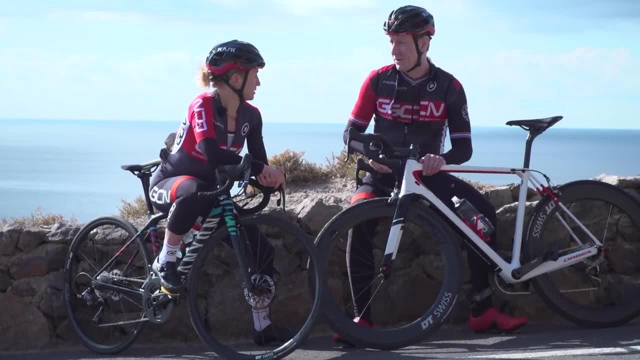 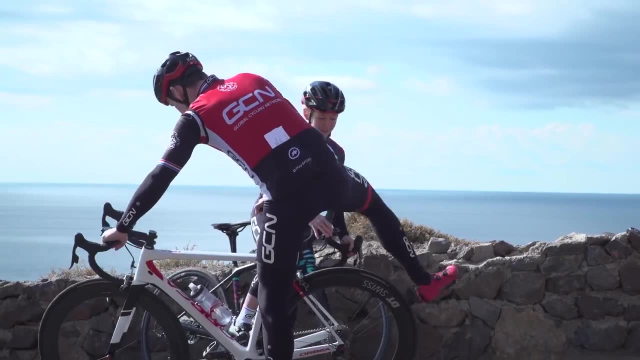 mistakes to avoid when climbing. Can we have some coffee and cake now? I'm absolutely ruined, Please. I'm knackered. That was ridiculous. Well, why did we choose such a steep hill? anyway, I thought it was going to be kind of a bit easier when you came to the channel. God, it's really hard. 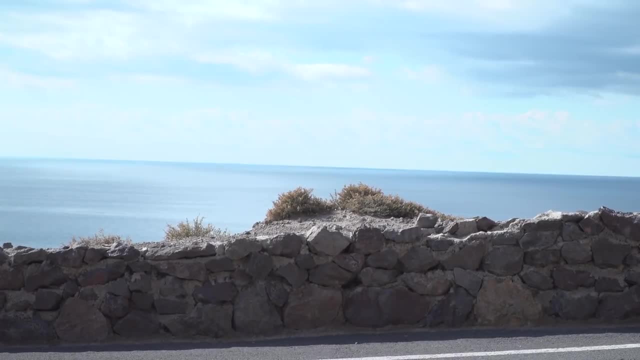 Well, can we choose some like flat sections or something, and I really I'm having a lot of problems clipping in. 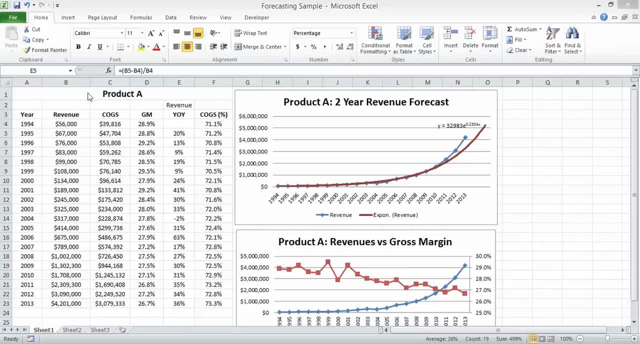 In this final video, using these data points for product A as an example. what I want to do is show you how you can create a nice little chart that charts out the year-over-year percentage increases or decreases for our revenues for product A for 1995 through 2013.. Just give you some tips and